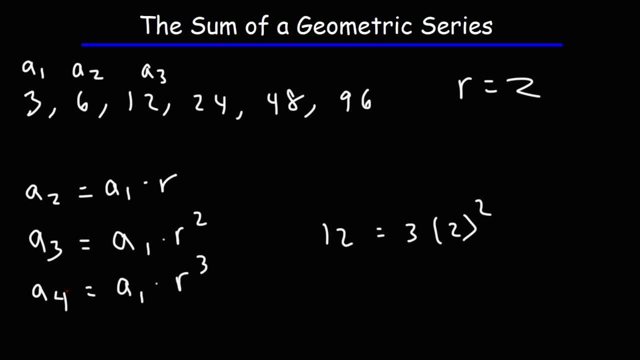 it's the first term. times r cubed 4 minus 1 is 3.. Make sure you understand that, because we're going to use that later to prove the formula. Now, what we have here is a sequence. To convert it into a series, we need to use the addition sign. 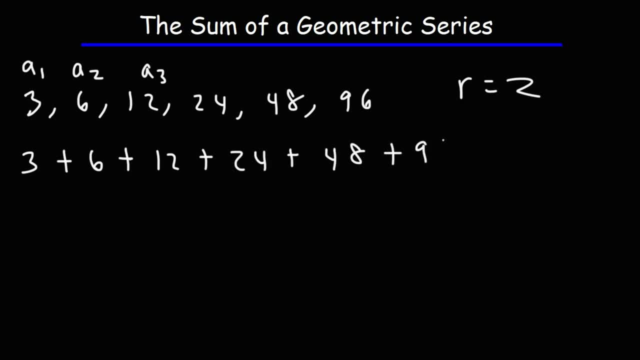 So this is a geometric series. So let's add up the first six terms. So this is going to be S6, the partial sum of the first six terms: 3 plus 6 plus 12 plus 24 plus 48 plus 96.. 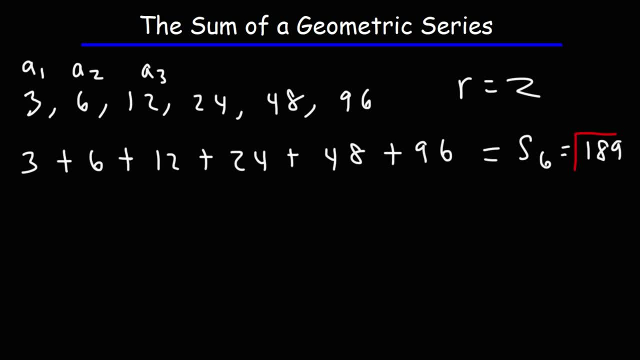 That's 189.. Now let's use the formula to calculate that sum. This is the formula that helps us calculate the sum. This is the formula that helps us to calculate the sum of a finite geometric series. It's a sub 1 times 1 minus r, raised to the n over 1 minus r. 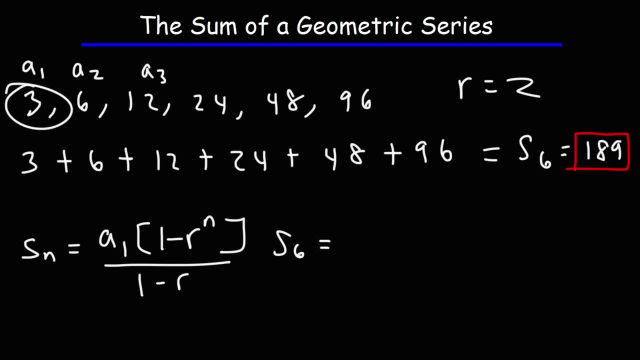 So to calculate, S6 is going to be a sub 1, the first term, which is 3, times 1 minus r, r is 2.. It's raised to the n. n is basically the number of terms, which is 6, over 1 minus 2.. 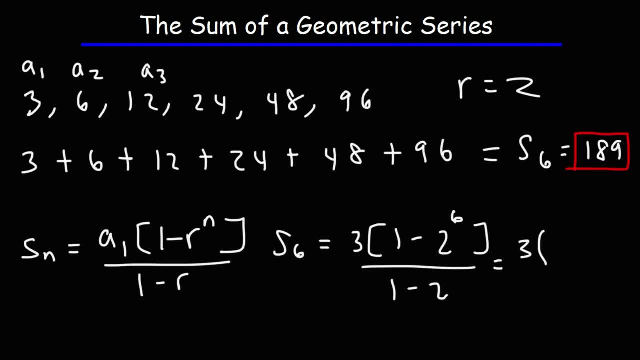 So this is going to be 3, 1 minus 2 raised to the 6th power. If you multiply 2 six times, you get 64.. 1 minus 2 is negative 1.. 1 minus 64 is negative 63.. 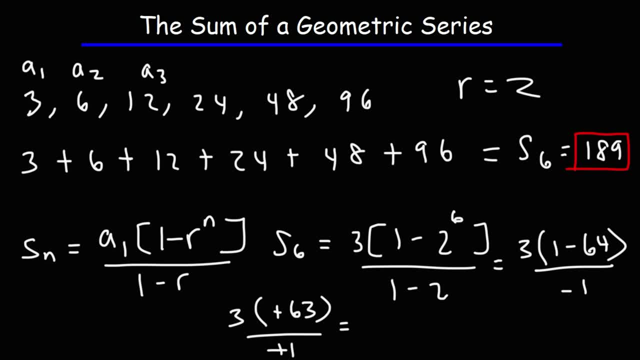 The two negative signs will cancel becoming positive. So it's 3 times 63.. 3 times 6 is 18.. 3 times 3 is 9.. So we get 189.. Which is the same as 1 minus 2.. 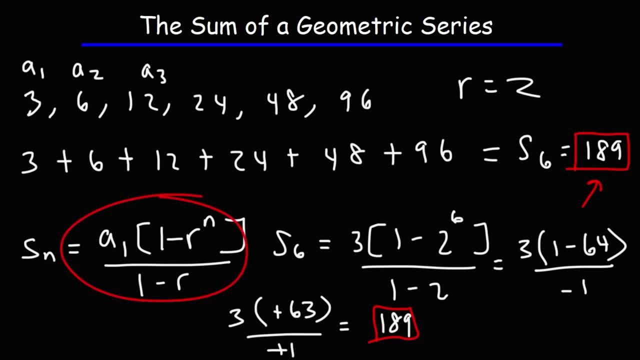 So this is the formula that helps us to calculate the sum of a finite geometric series. Now what if we were to have an infinite geometric series? So let's say we have the series 8 plus 4 plus 2 plus 1 plus 1 half plus 1 fourth. 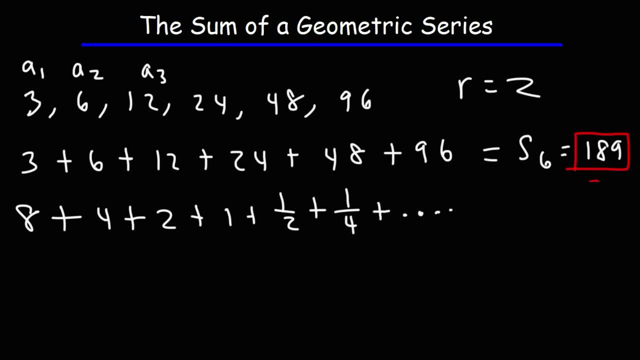 And then plus dot dot dot. So this series here, it has a beginning and it has an end, So it's a finite geometric series. This series doesn't have an end, It goes on forever, So it's an infinite geometric series. 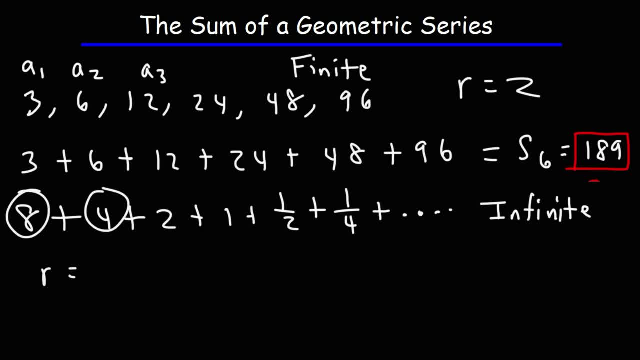 The common ratio, if you take the second term divided by the first, 4 divided by 8, is 1 half. The common ratio is 1 half for all terms Now, because the common ratio, or rather the absolute value, is the absolute value of r. 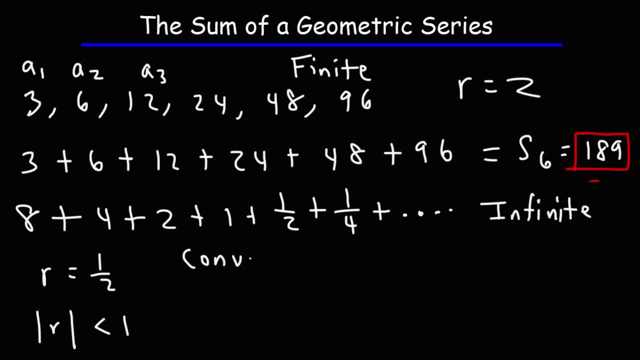 because it's less than 1, the series converges, which means that the sum is finite. If the absolute value of r, if it was greater than 1, the series would diverge and you wouldn't be able to calculate the sum. 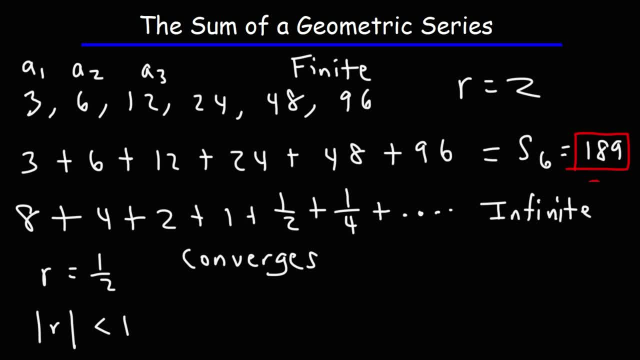 Because it can increase towards positive or negative infinity. So it's important that the common ratio, the absolute value of the common ratio, be less than 1 for this to work. And the sum of this infinite geometric series, we can write s sub infinity. 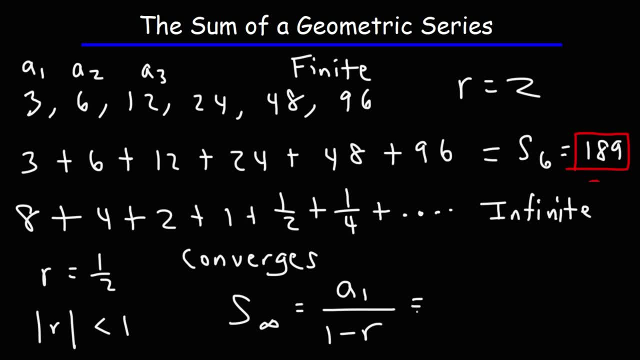 it's the first term- divided by 1 minus r. So in this example it's 8 over 1 minus 1 half. 1 minus 1 half is 1 half 8 divided by 1 half, If you multiply the top and the bottom by 2,. 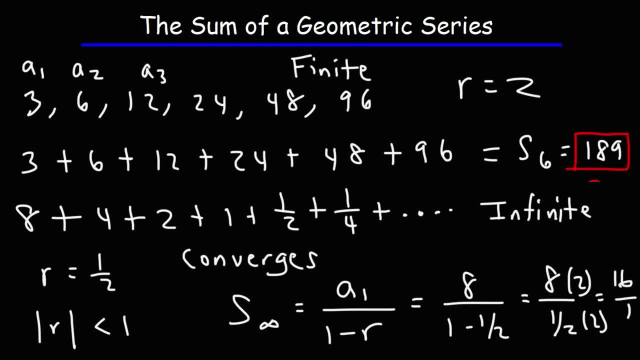 this becomes 16 over 1, which is 16.. So if you were to add these numbers, 8 plus 4 is 12. Plus 2,, that's 14. Plus 1, 15. Plus 1, half 15.5.. 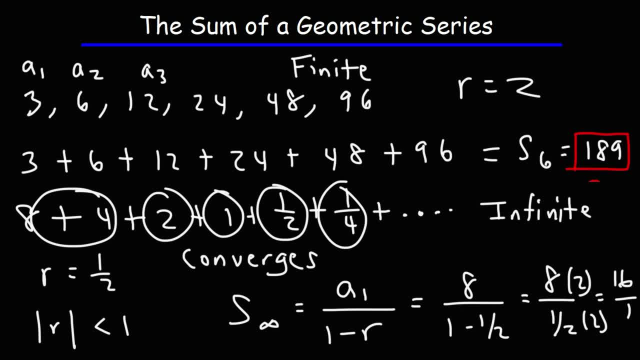 Plus 1, 4,, 15.75.. If you keep doing this, you're going to get closer and closer to 16.. But you're not going to pass 16.. So that's the sum of this infinite geometric series. Now let's talk about 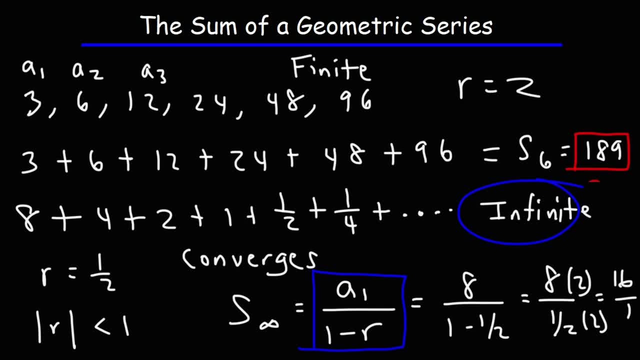 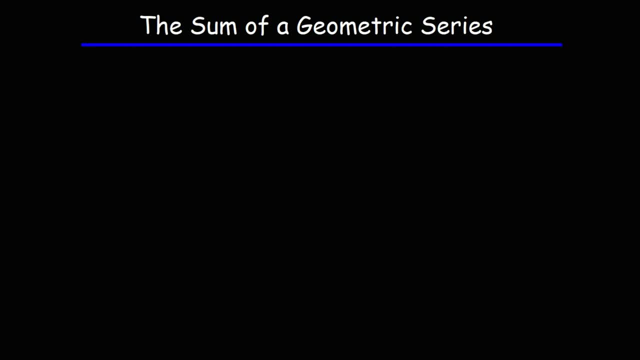 how to prove this formula as well as the other one. So let's start with the formula that describes the sum of a finite geometric series. So we're going to have s sub n is a1 plus a2 plus a3 plus a4, and then the 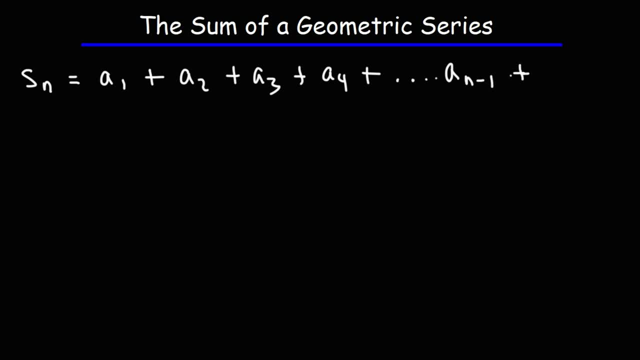 second to last term is minus 1, and the last term will be a sub n, Now a sub 2, recall that a sub 2 is a sub 1 times r And a sub 3, we said that it's a sub 1 times r, squared. 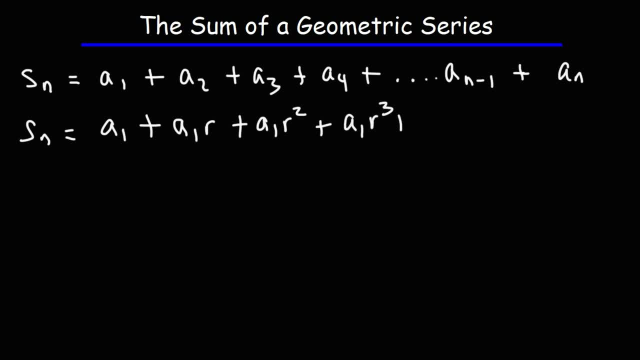 a4 is a sub 1 times r cubed. By the way, the formula that describes the nth term of a geometric series or a geometric sequence is a sub 1 r raised to the n minus 1.. So in our first example we had the series: 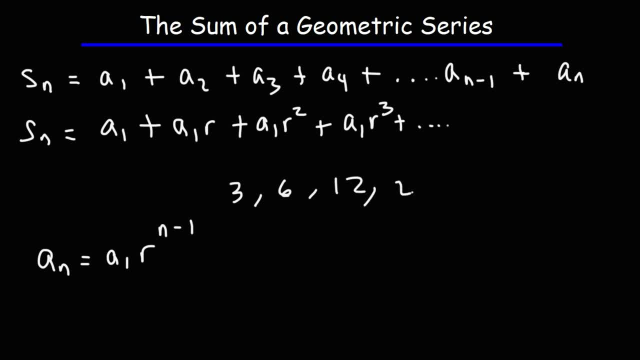 or the sequence 3, 6,, 12,, 24, 48.. Let's say, if we want to calculate the fifth term, It would be: a sub 5 is equal to a sub 1, which is 3 times r. r is 2. 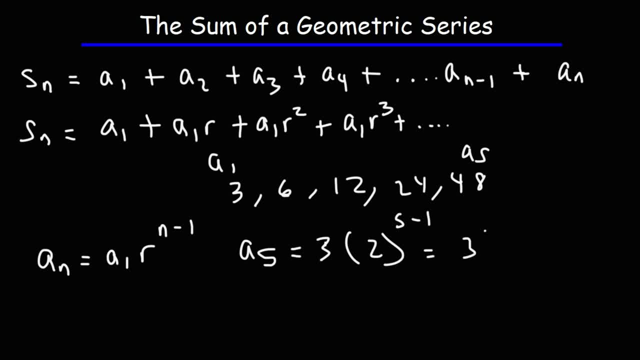 raised to the n minus 1 or 5 minus 1.. 5 minus 1 is 4.. 2 to the fourth power: 2 times 2 times 2 times 2, that's 16.. 3 times 16: 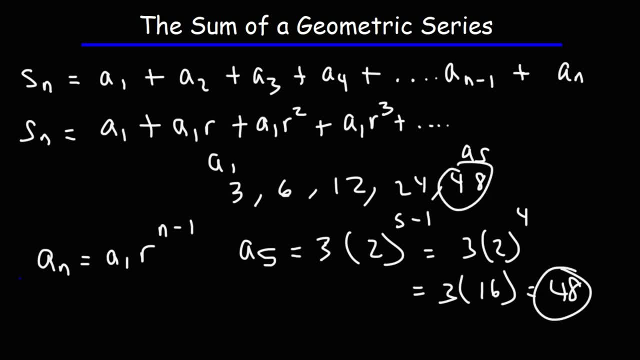 is 48. So this formula here gives you the nth term of a geometric sequence. So let's think about that. If a sub n is a sub 1 times r raised to the n minus 1, what is a sub n minus 1?? 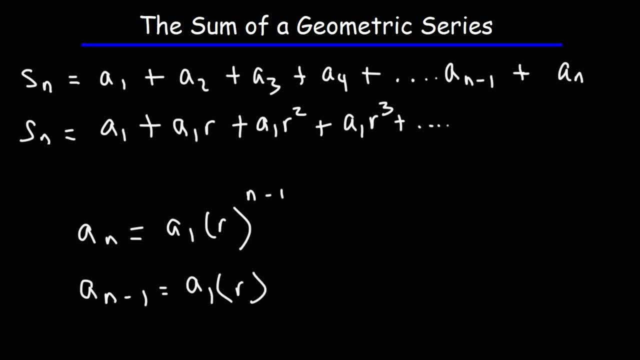 a sub n minus 1 is going to be a sub 1 times r, but we're going to plug in n minus 1 into that expression, So replace an n with n minus 1.. We get a sub 1 r raised to the n minus 2.. 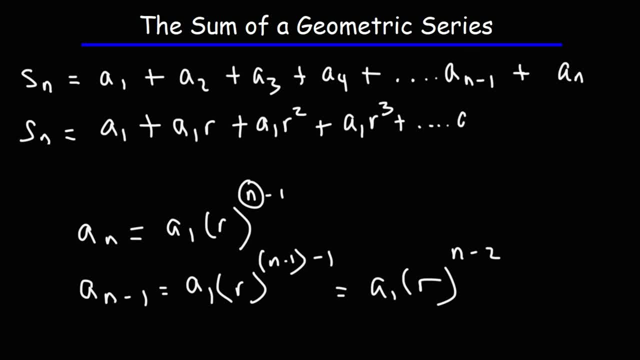 And that's what we're going to replace this thing with. It's going to be a sub 1 r to the n minus 2.. And then a sub n. we already have that here. That's just a sub 1 r to the n minus 1.. 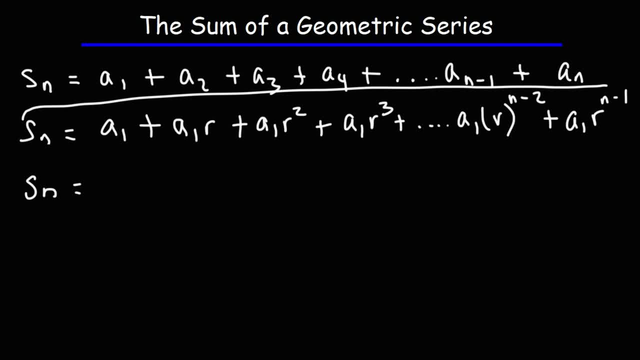 Now for the next line. what we're going to do is we're going to take this equation and we're going to multiply it by r. So this is going to be r s n, and then this is going to be a sub 1 times r. 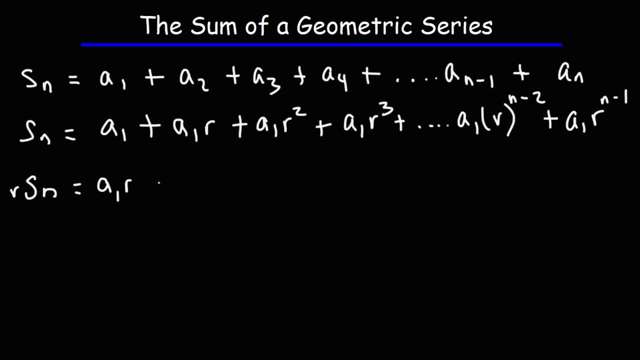 This becomes if you multiply by r. it's going to be a sub 1 r squared, and then plus a sub 1 r cubed, plus a sub 1 r to the fourth, and then, multiplying this by r, the exponent is going to increase by 1.. 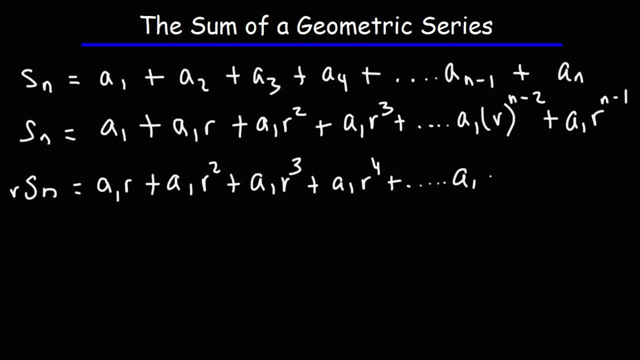 So n minus 2 plus 1, that's going to be n minus 2 minus 1.. Multiplying this by r, the exponent will increase by 1 as well. so n minus 1 plus 1 becomes simply n Negative 1 and positive 1 will cancel. 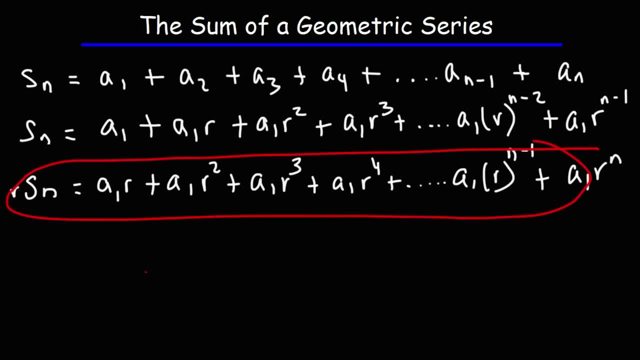 Now what we're going to do is we're going to multiply this equation by negative 1.. So this is going to be negative, and then every term within the bracket, once we distribute the negative sign will be negative. So now we're going to add: 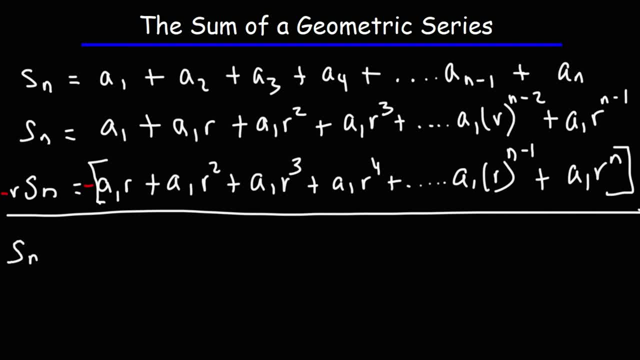 these two equations. So we're going to have s sub n plus negative r s sub n, or simply s sub n minus r s sub n, and then we'll have a 1, Now, a 1 r minus a 1 r. they're going to. 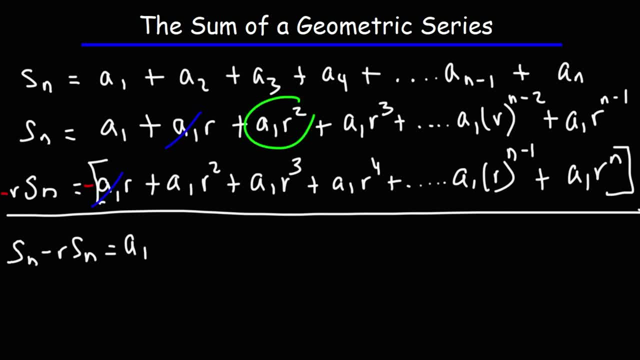 cancel a 1 r squared minus a 1 r squared, they will cancel as well a 1 r. cubed is going to cancel. a 1 r to the fourth will cancel with something that's here and then a 1 r n minus 2. 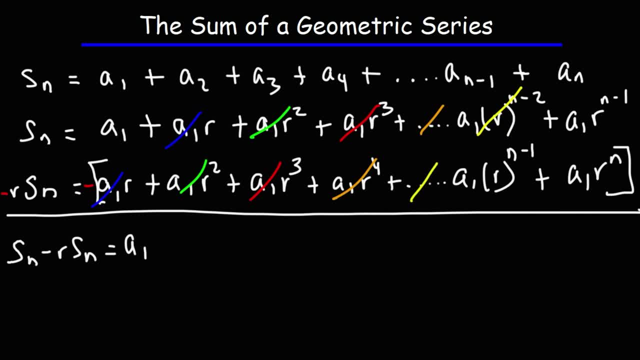 will cancel with something that's there, and then a 1 r n minus 1 will cancel as well. This one will not cancel, but it has a negative sign. so it's going to be negative. a 1 r raised to n. Now what we're going to do? 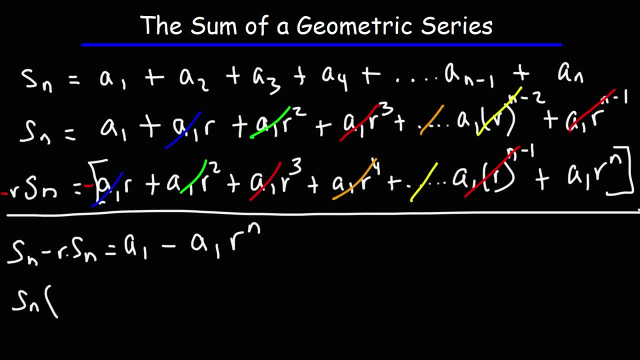 is we're going to factor out s sub n. s sub n divided by itself is 1. negative r. s sub n divided by s sub n is going to be negative r. Here we're going to factor out a sub 1 divided by itself is 1. 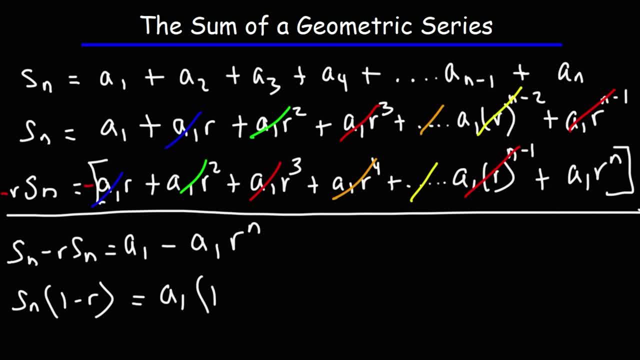 negative a. 1 r to the n divided by a 1 is negative r raised to the n. and then we're going to divide by 1 minus r. So this gives us the formula for the partial sum of a finite geometric series. It's the first term. 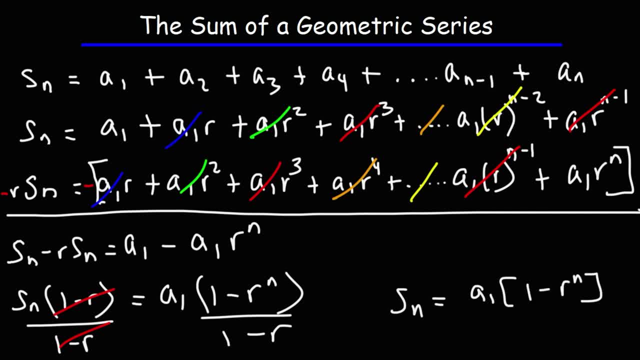 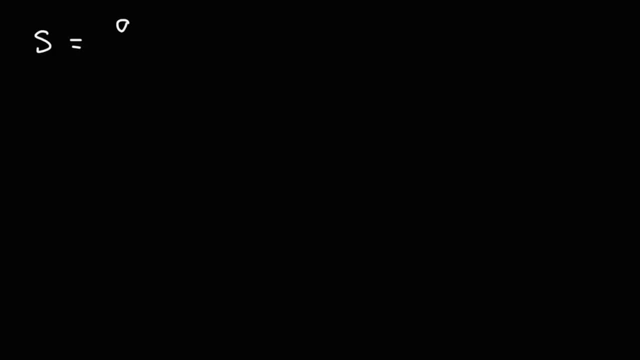 times 1 minus the common ratio raised to the n over 1 minus r. So that's how we can derive the sum of a finite geometric series. Now let's talk about how we can get this formula. In order to get that formula, we need to realize: 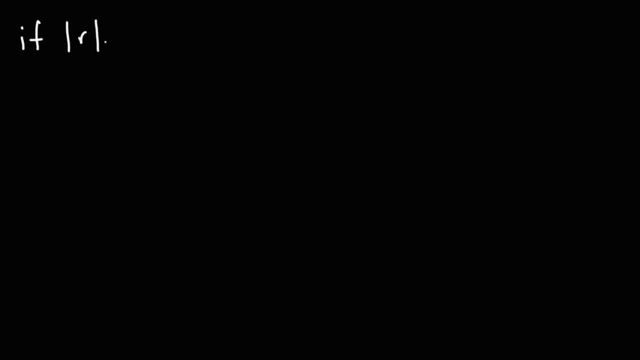 that if the absolute value of r is less than 1 and as n goes to infinity, r raised to the n, it goes to 0, not infinity. Now let's talk about that. So if we have 0.9, which is less than 1, raised to the first power, 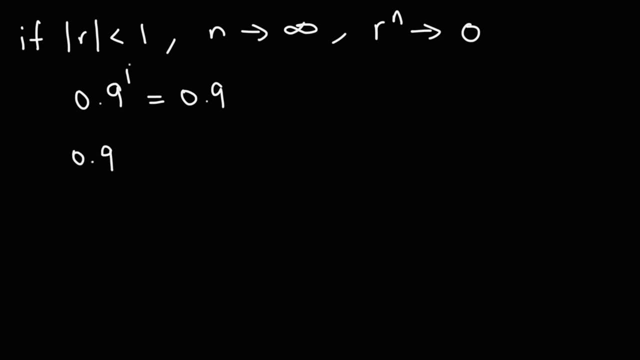 that's 0.9. But what happens if we increase the exponent from 1 to 10? Will this number get bigger or lower? 0.9 raised to the 10th power is a smaller number: 0.348678. Let's use. 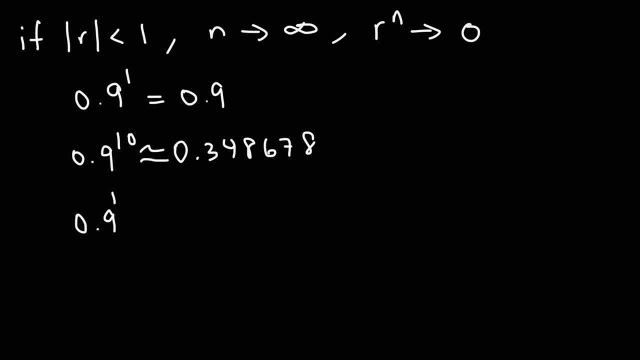 the approximate symbol. Now let's increase it to 100: 0.9. raised to 100, It's even smaller. It's 0.0002656, 0.0002656, 0.0002656, 0.0002656. So we can see that.